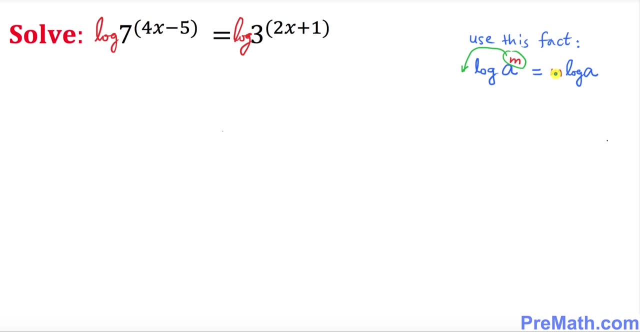 Okay, like I did this one over here, So m is going to show up at the front And then you put a log on this side And then you put a log of a, In our case over here. as you can see, over here we have right now, over here we have. this is our exponent. 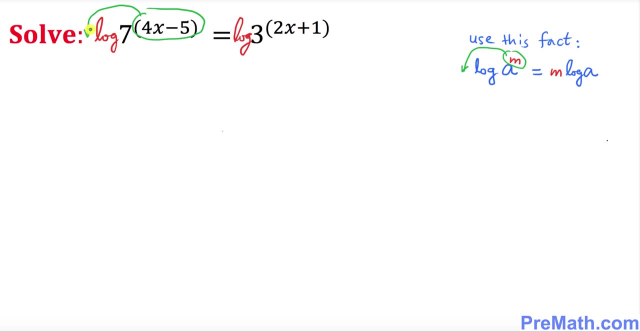 So this exponent is going to show up, is going to show up at the beginning. Likewise, this exponent is going to show up in the front. So what that means is our problem is going to look like this one. So this exponent, I want you to put it in the front. 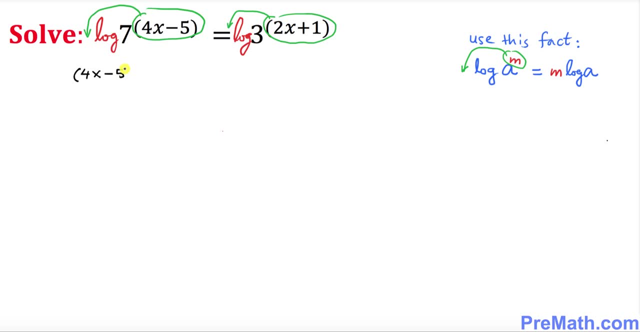 4x minus 5 outside, Then this becomes log of 7, equal to same thing, This exponent. you move it at the front: 2x plus 1 log of 3.. Now one more thing. As you can see over here, if you use a calculator, log of 7 is approximately equal to 0.85. 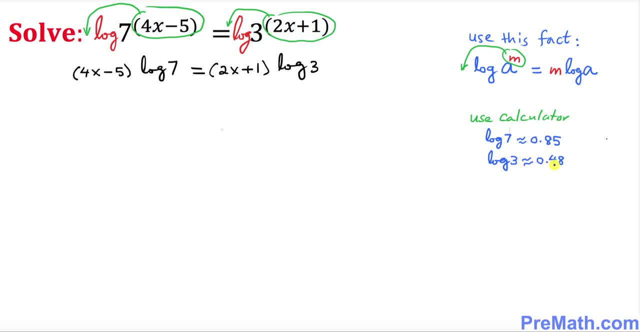 And log of 3 is approximately equal to 0.48.. So wherever you see log of 7, I'm going to replace it by that quantity, that amount. So I'm going to put down 4x minus 5 times log of 7 is 0.48. 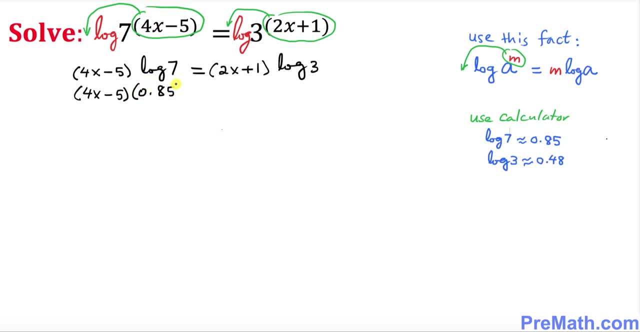 So log of 7 is 0.85, equals to 2x plus 1.. And log of 3 is 0.48.. Now the next thing, what I want you to do, is go ahead and multiply it out, distribute it. 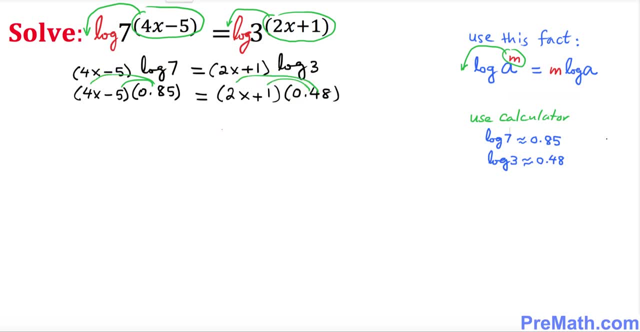 Likewise, you multiply it out over here. Once you multiply it out over here, 4x times 0.87 is going to give us 3.4x minus 4.25 on the left-hand side equals to Now you're going to multiply 2x. 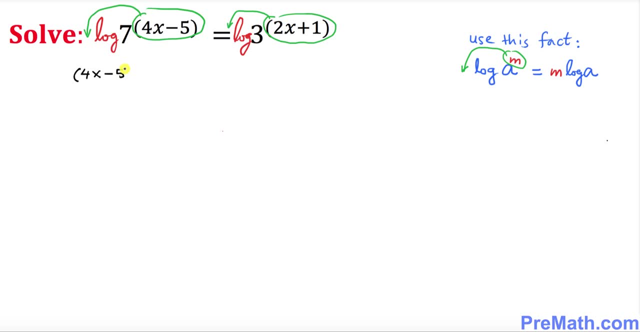 4x minus 5 outside, Then this becomes log of 7, equal to same thing, This exponent. you move it at the front: 2x plus 1 log of 3.. Now one more thing. As you can see over here, if you use a calculator, log of 7 is approximately equal to 0.85. 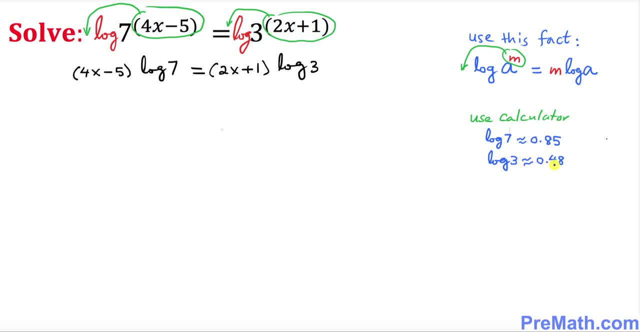 And log of 3 is approximately equal to 0.48.. So wherever you see log of 7, I'm going to replace it by that quantity, that amount. So I'm going to put down 4x minus 5 times log of 7 is 0.48. 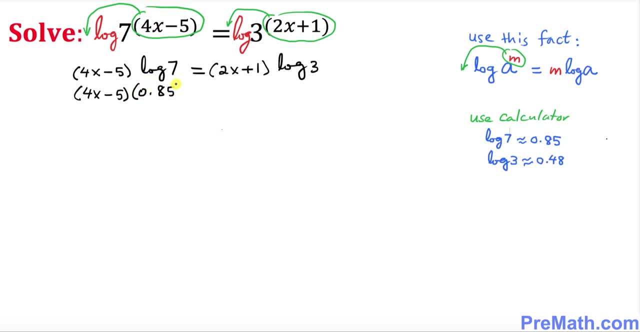 So log of 7 is 0.85, equals to 2x plus 1.. And log of 3 is 0.48.. Now the next thing, what I want you to do, is go ahead and multiply it out, distribute it. 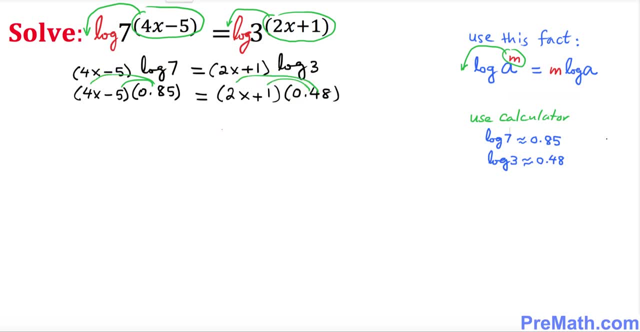 Likewise, you multiply it out over here. Once you multiply it out over here, 4x times 0.87 is going to give us 3.4x minus 4.25 on the left-hand side equals to Now you're going to multiply 2x. 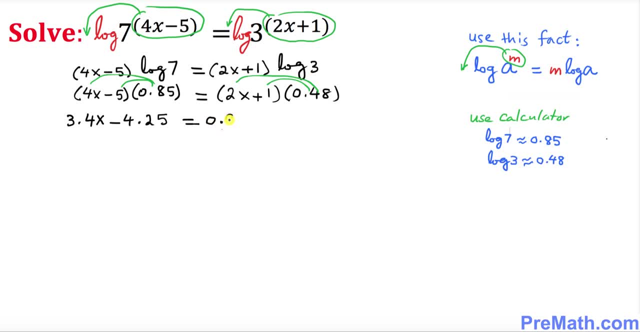 4x times 0.48 is going to give you 0.96x plus 0.48.. Now the next step is I want you to combine the like terms: Move x's on one side and the non-x's constant on one side.